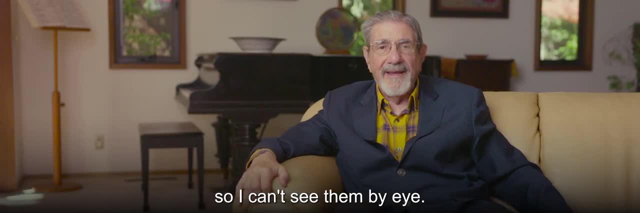 So molecules aren't that big, so I can't see them by eye. However, I can do something to them to make them so you can see them. One of the things I can do is I can see them by eye. One of the things I can do is I can excite them with a laser and make them fluoresce. 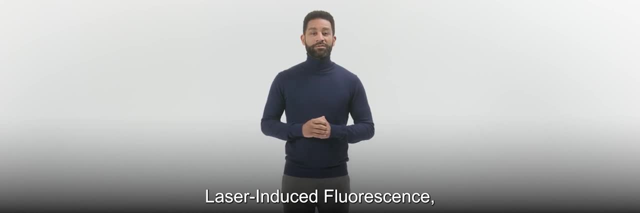 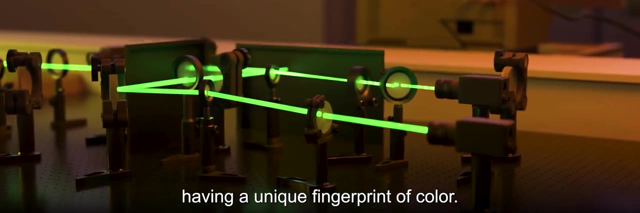 Fluoresce To glow. Laser-induced fluorescence, or LIF, excites molecules with a laser beam and then measures the light they give off, each molecule having a unique fingerprint of color With a self-built laser, Zare ignited a revolution. 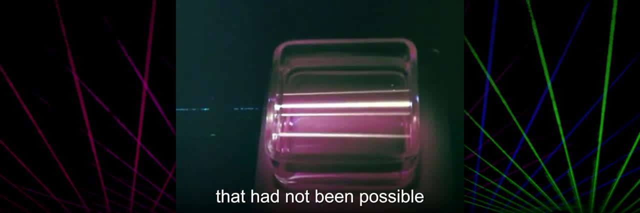 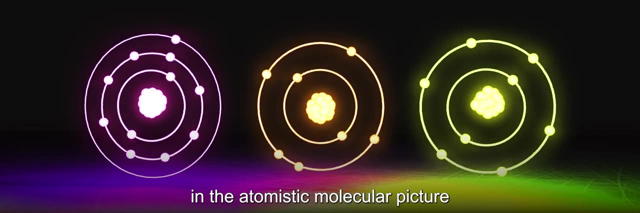 We could see things at a level that had not been possible to be seen before, and it certainly made one believe that they were real. We could see things at a level that had not been possible to be seen before, and it certainly made one believe that they were real. 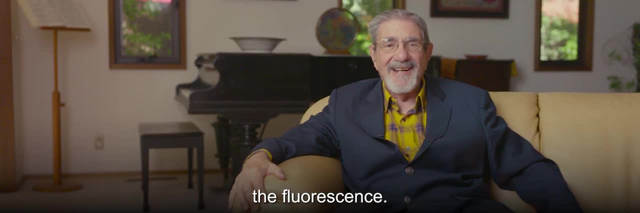 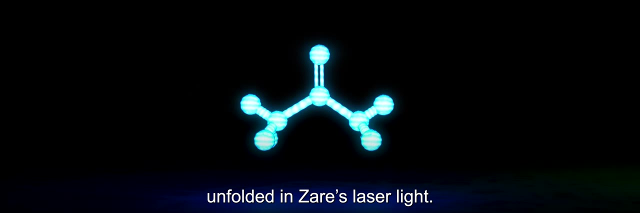 We could see things at a level that had not been possible to be seen before, and it certainly made one believe that they were real. Suddenly, we could actually see the shapes of molecules, witness their evolutions as chemical reactions unfolded in Zare's laser light. 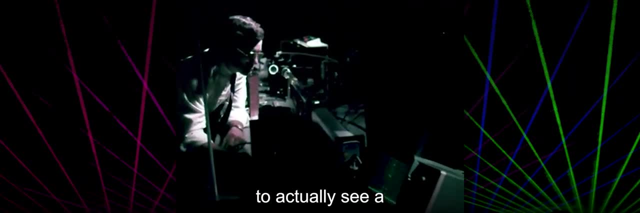 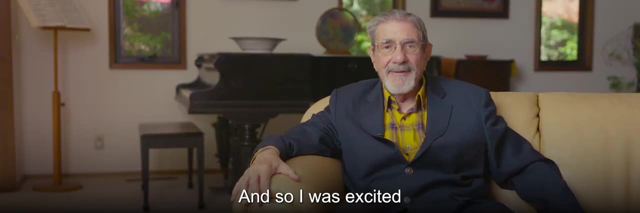 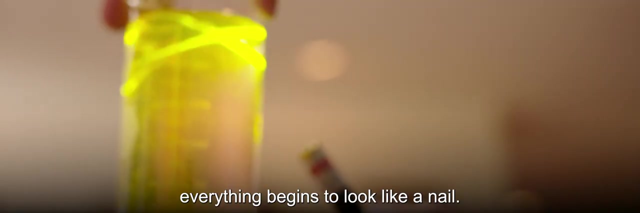 We would actually, I think, be the first people to actually see a single molecule at room temperature in a liquid actually fluoresce and detect it, And so I was excited about those possibilities, And those possibilities seemed endless. Zare's motto: Once you have a hammer, everything begins to look like a nail. 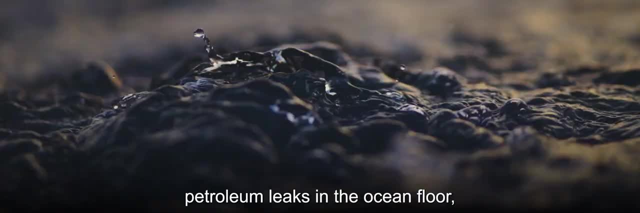 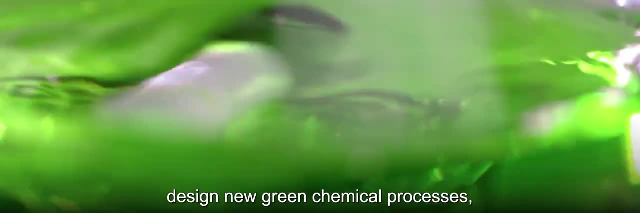 Over the decades, LIF has been used to discover petroleum leaks in the ocean floor, detect cancer, reduce carbon emissions, determine the age of ancient artifacts, design new green chemical processes, and even led to one of the greatest achievements of the 20th century. 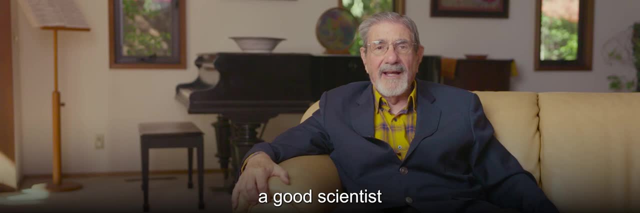 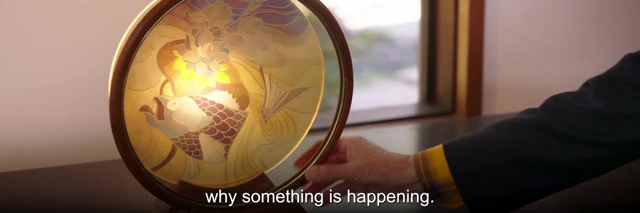 the sequencing of the human genome. I actually think a good scientist who believes and disbelieves at the same time. You've got to believe and put forward an idea why something is happening And after you put forward that idea you've got to turn around and say: is that really so? 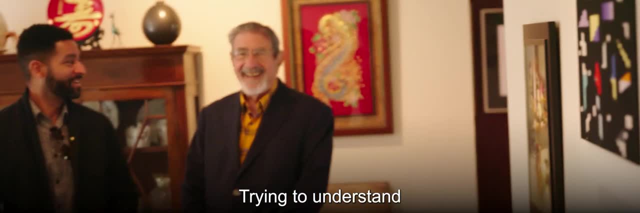 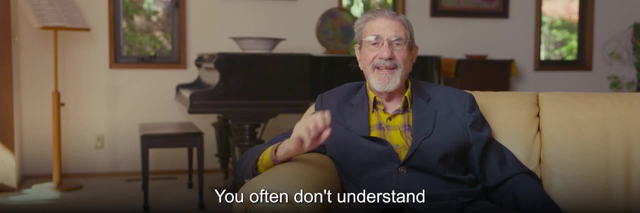 Is that true And question it, Trying to understand why things are the way they are- A belief, really, that there can be an explanation for what you're seeing. You often don't understand the power of the question. It's actually more important than the answer.